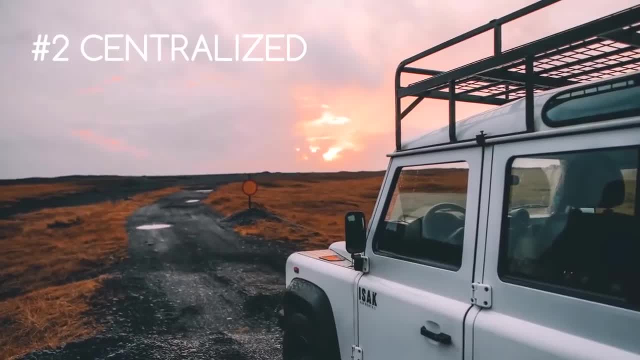 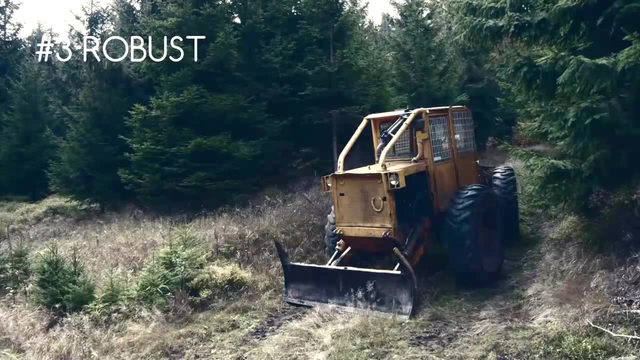 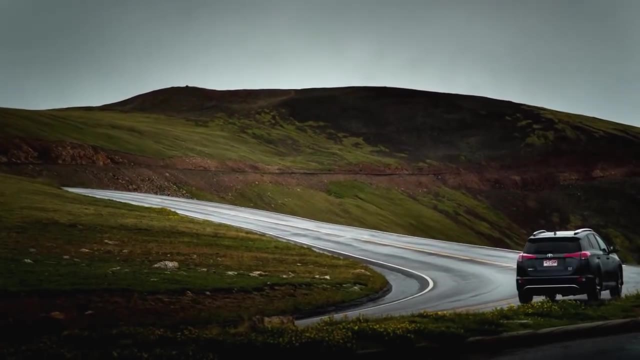 Two: centralized: The Canbus system allows for central error diagnosis and configuration across all ECUs. Three: robust: The system is robust towards failure of subsystems and electromagnetic interference, making it ideal for, in example, vehicles. Four: efficient: 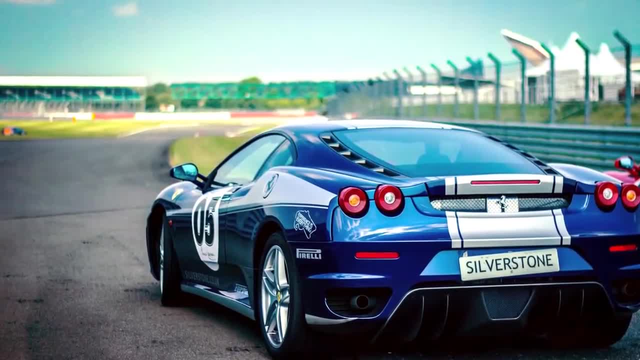 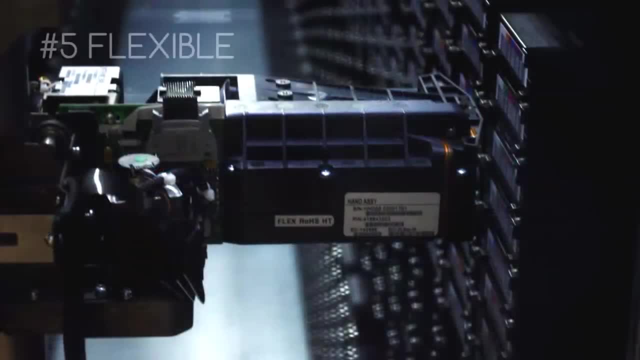 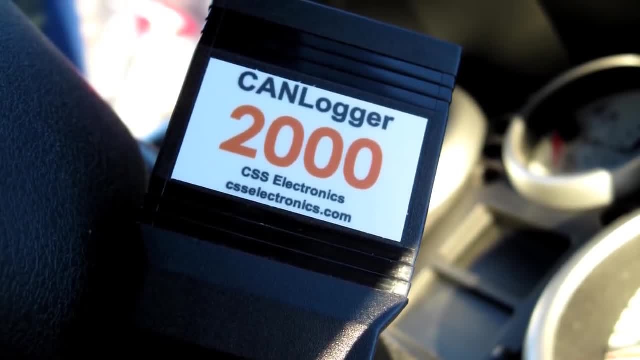 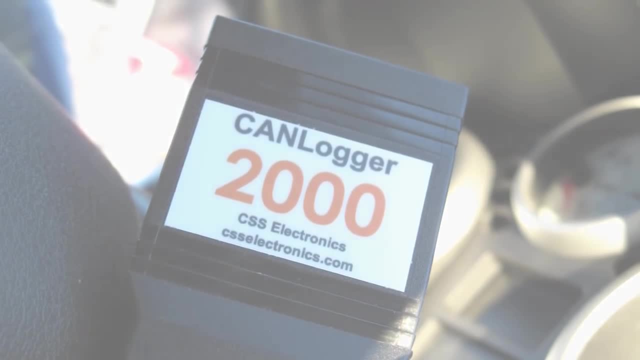 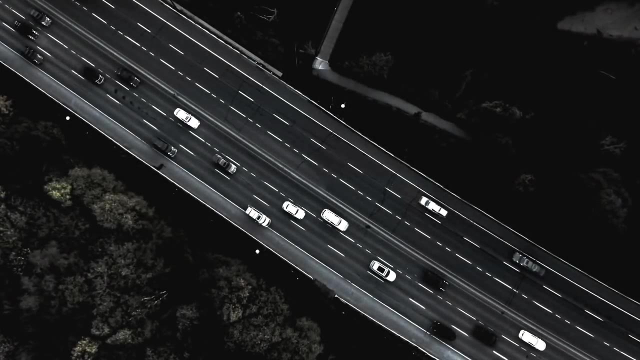 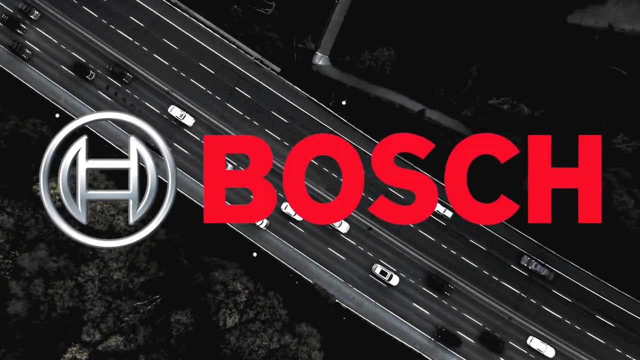 all transmitted messages, decide relevance and act accordingly. This allows easy modification and inclusion of additional nodes such as Canbus data loggers. The Canbus history, in short. Pre-Can car ECUs relied on increasingly complex point-to-point wiring. 1986, Bosch developed the CAN protocol as a solution, releasing it at a SAE Congress. 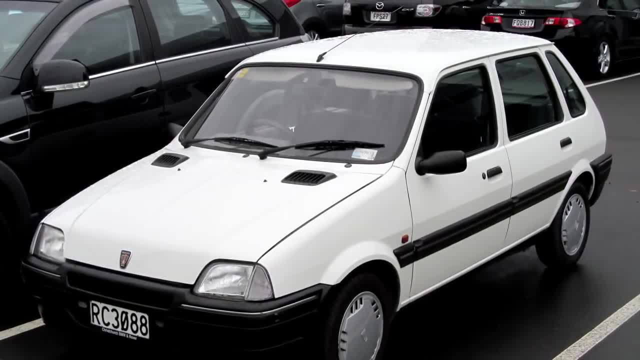 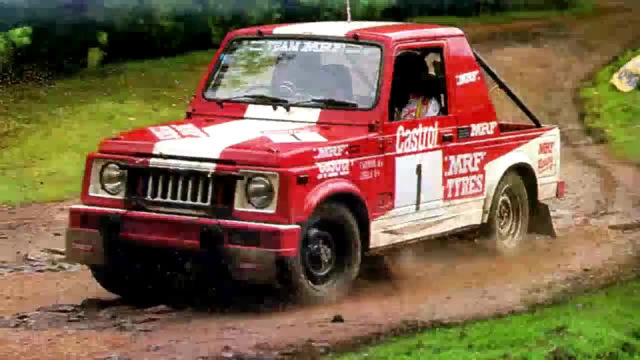 1991, Bosch published CAN 2.0, Inclusion CAN 2.0a 11-bit and CAN 2.0b 29-bit. 1993, CAN is adopted as international standard ISO 1189-8.. 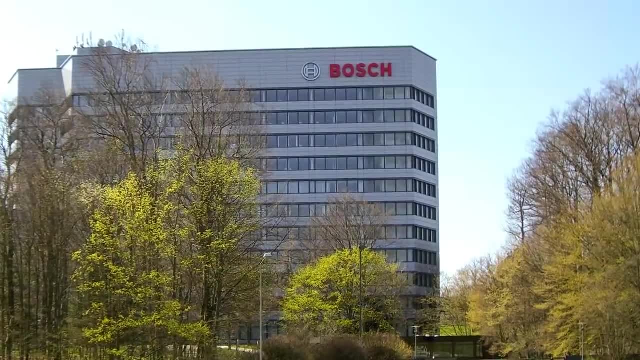 2000,. Can is adopted as international standard: ISO 1189-8.. 2000,. Can is adopted as international standard: ISO 1189-8.. 2012,. Bosch released the CAN FD 1.0, aka CAN, with flexible data rate. 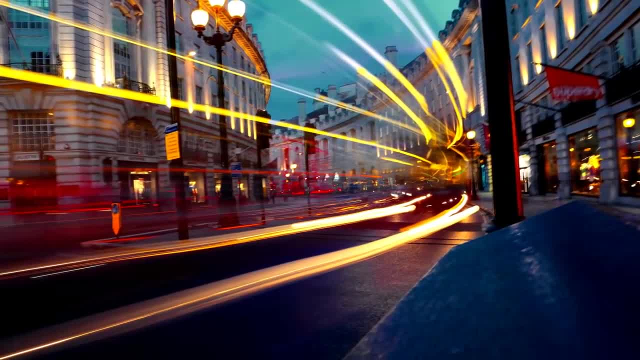 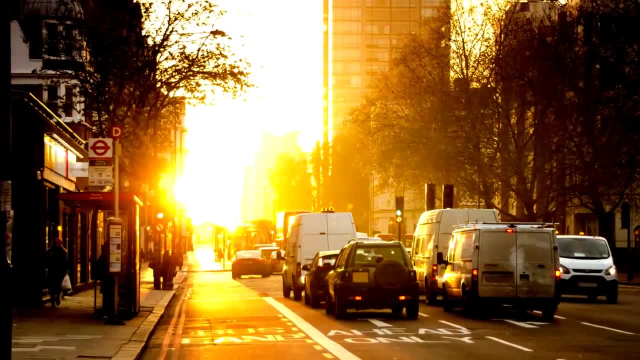 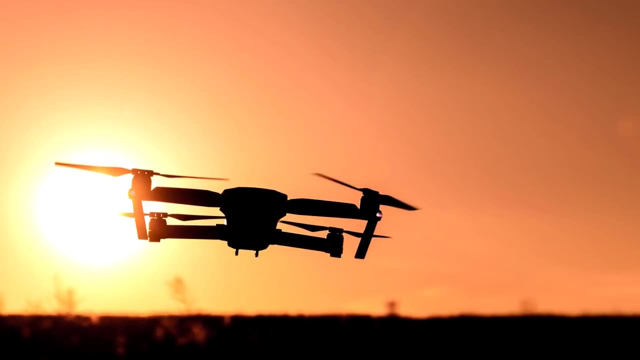 Today, almost every new European car comes with a CAN bus system, and it is used broadly in trucks, buses, industry vehicles, ships, planes and industrial automation. Further more exotic cases include drones, radar systems, submarines or even prosthetic limbs Looking. 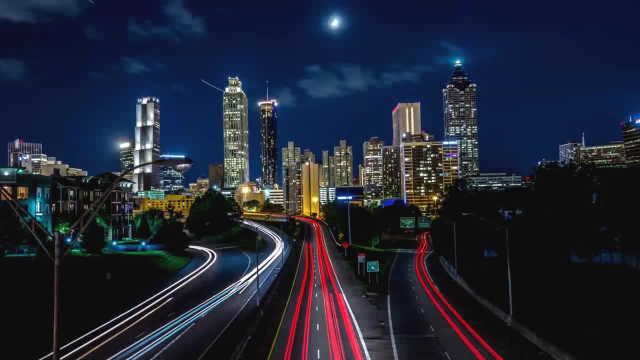 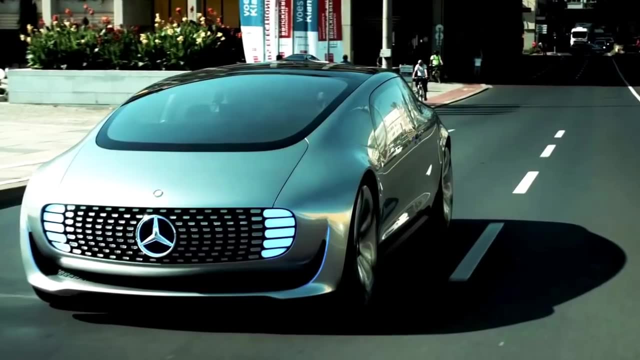 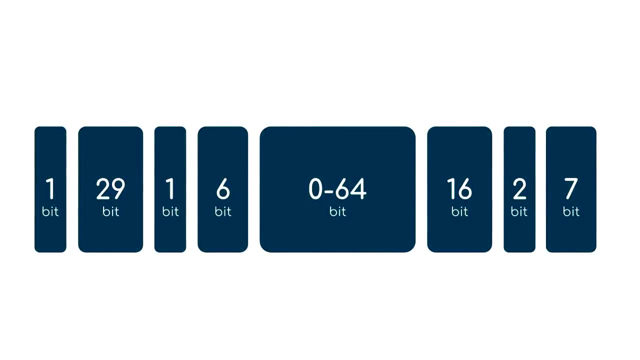 ahead. the CAN bus system will stay relevant And most likely even more so with the rise of, example, cloud computing, Internet of Things, IoT and autonomous vehicles. What does a CAN message look like? To understand how the CAN bus system works, let's break down the messages sent over. 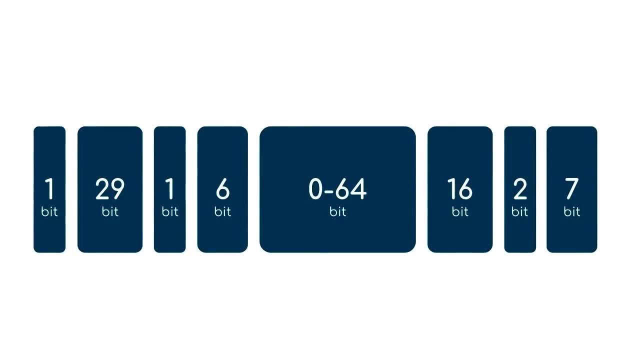 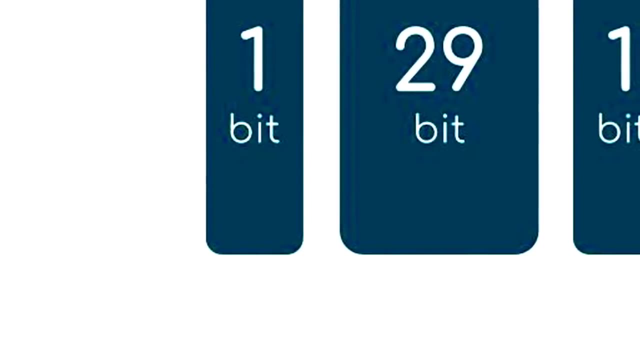 the network The 11-bit identifier CAN 2.0a messages look similar but with shorter CAN IDs. The eight key parts of a CAN message are as follows: SOF: The start of frame is a dominant zero to tell the other ECUs that a message is coming. 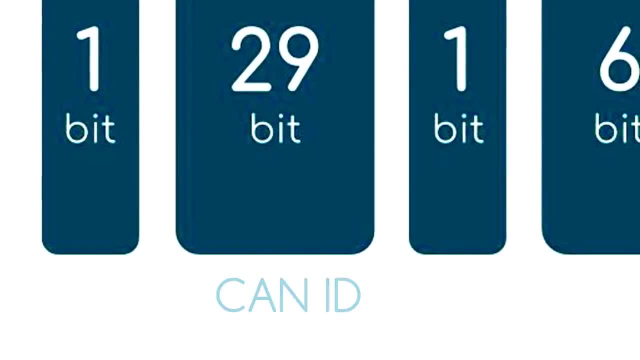 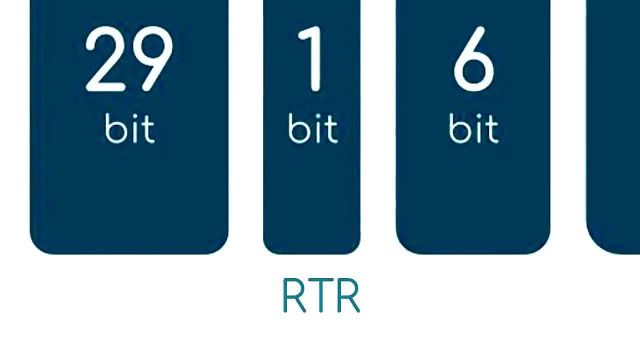 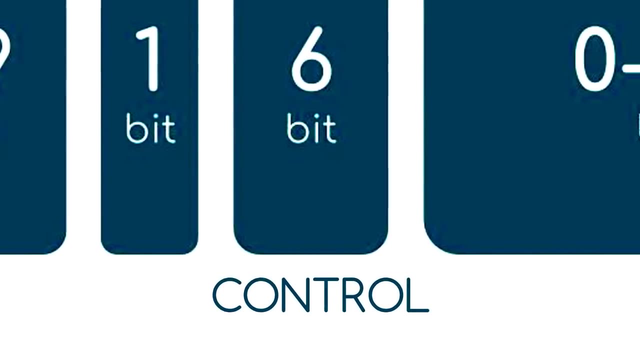 CAN ID contains the message priority as well as functional address. an example: RPM, wheel speed, RTR. the remote transmission request allows ECUs to request messages from other ECUs. Control informs the length of the data in bytes, zero to eight bytes. 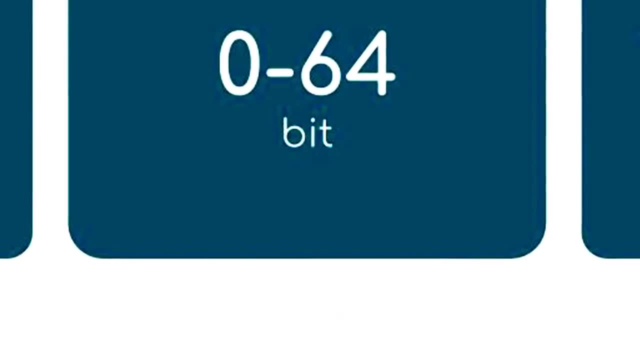 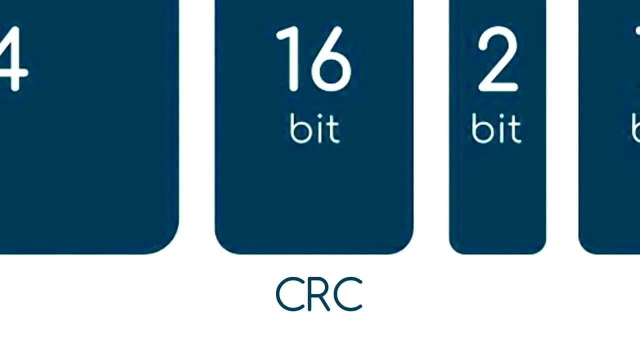 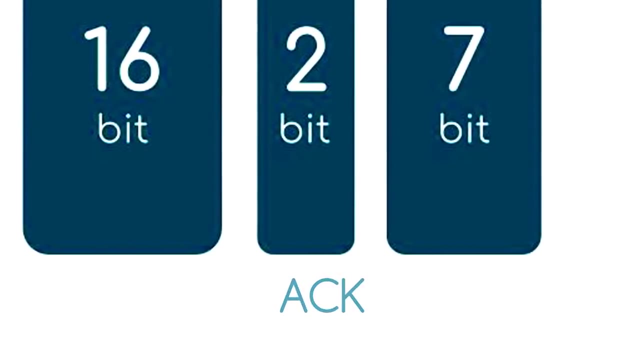 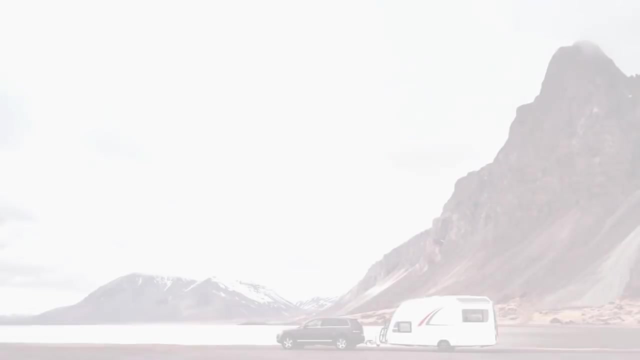 Data contains the actual data values which need to be scaled or converted to be readable and ready for analysis. CRC, The cyclic redundancy check, checks data integrity. ACK, The new dot-can-catch property slot, indicates if the CRC process is ok. EOF- 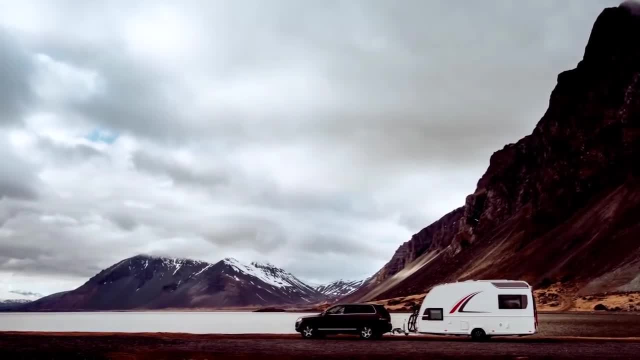 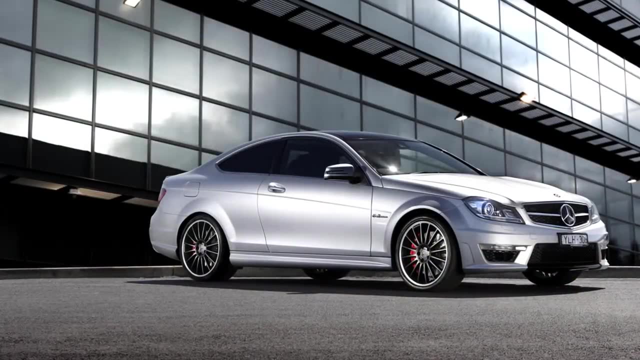 Marks the end of the CAN message. That's a lot, But only three are practically relevant in most data logging scenarios: The CAN ID, The control And the data field. This is also why you typically only see these in CAN bus data output. 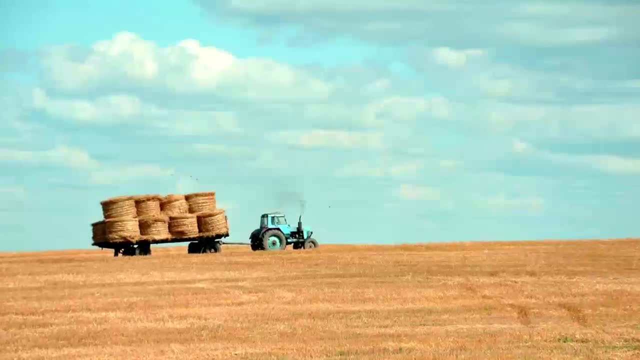 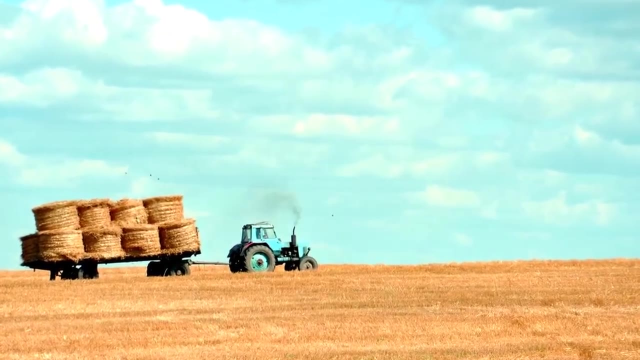 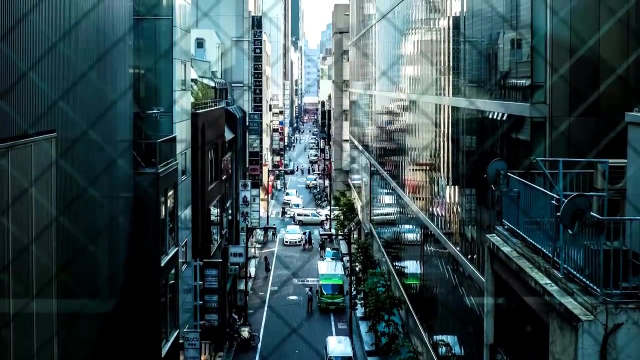 CAN provides the basis for communication, but not a lot more larger than 8 bytes or how to decode the raw data. Therefore, a set of standardized protocols exists to further define how data is communicated between ECUs of a given network. Some of the most commonly encountered standards include SAE J1939,. 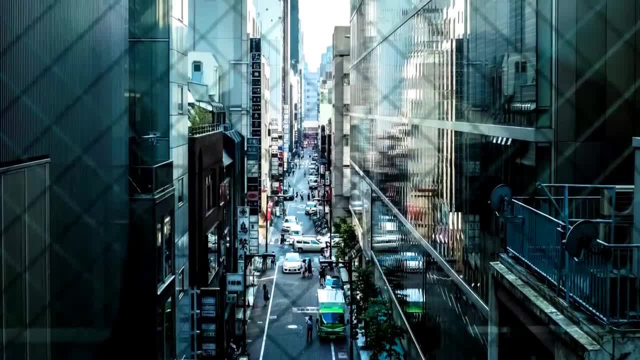 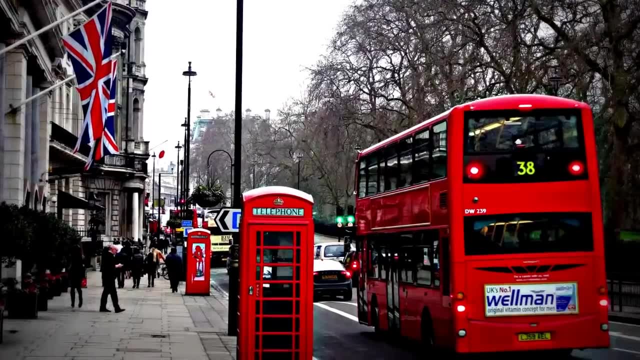 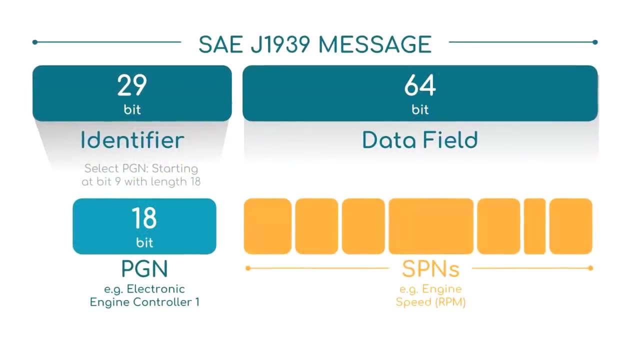 OBD2, and CANopen SAE J1939.. This is the standard in vehicle network for buses, trucks and other heavy-duty vehicles. All J1939 messages rely on the extended 29-bit CAN identifier. Further J1939 data parameters. 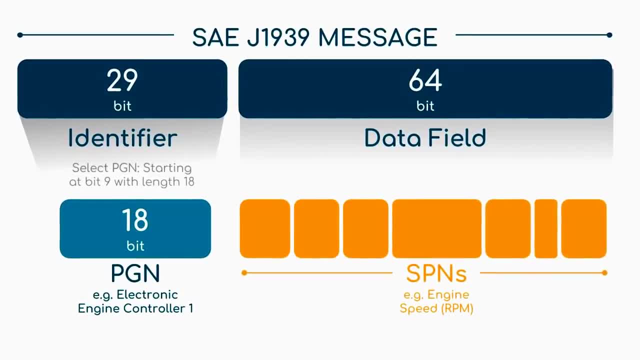 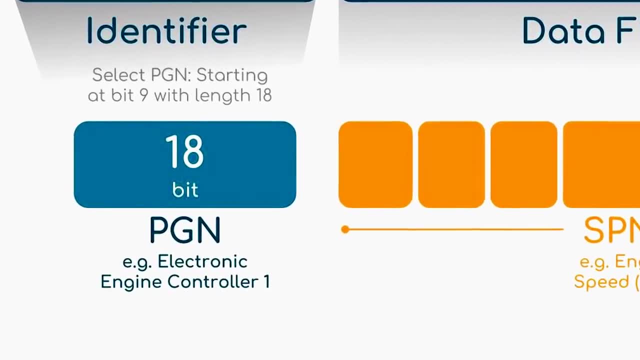 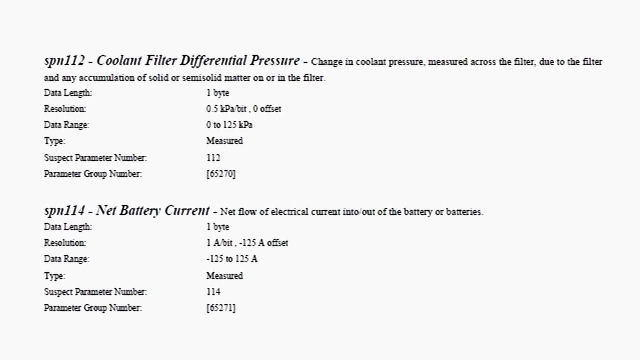 are identified by a suspect parameter number, which are in turn grouped in parameter group numbers containing 1 plus SPNs. With this standardized structure, CAN messages from example buses and trucks can be scaled and decoded into readable data using parameter tables from the J1939. 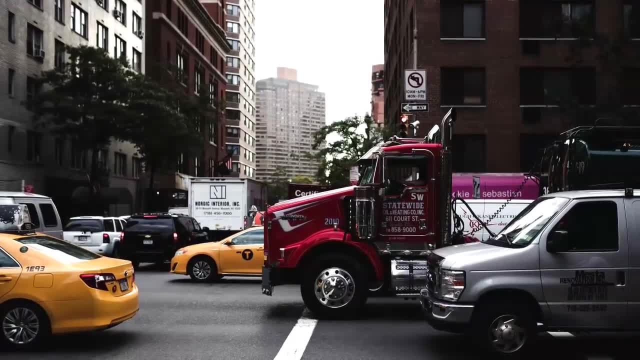 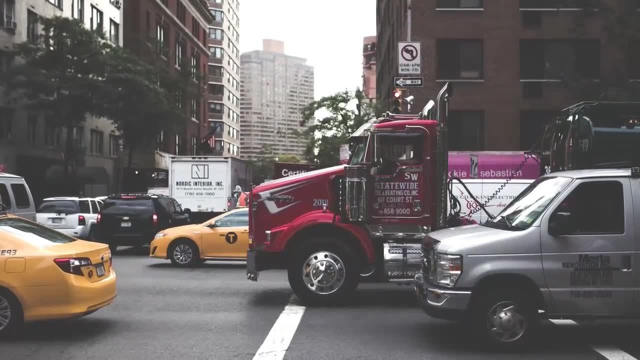 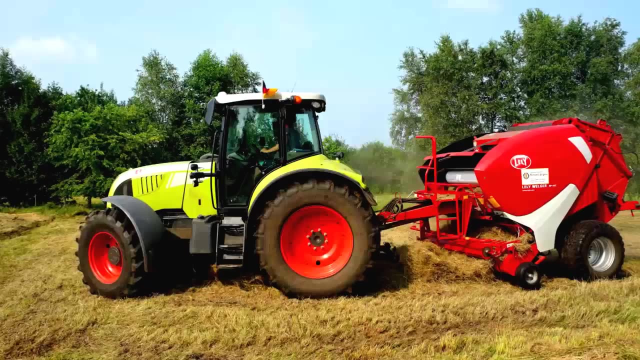 standard. Further, several standards are derived from J1939, including, in example, the Fleet Management System which is freely available and included in CANvas. For more information, see our simple intro to J1939, or our J1939 ID to PGN converter. 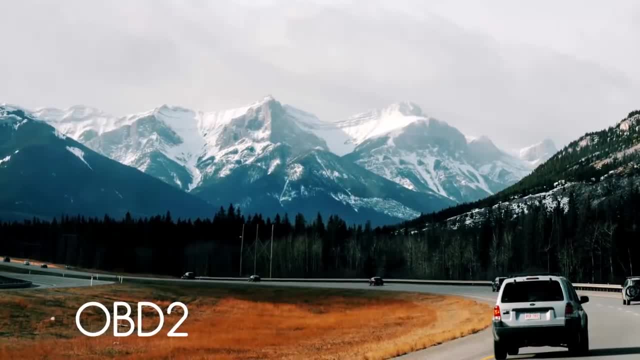 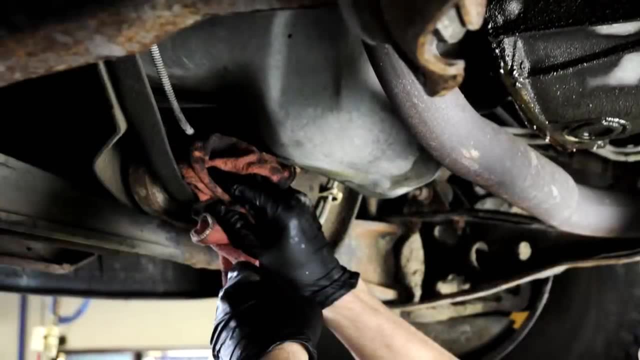 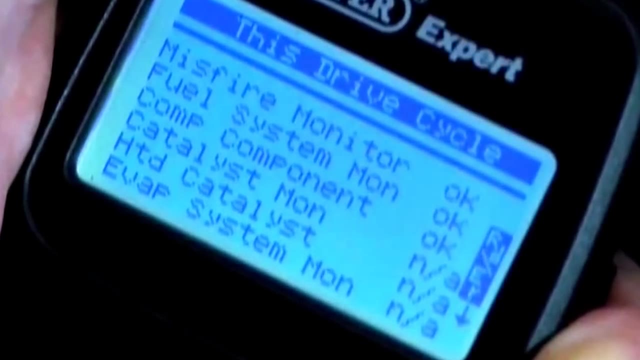 OBD2.. On-board diagnostics is a self-diagnostic and reporting capability that, in example, mechanics use to identify what is wrong with your car. The OBD2 standard specifies a number of standardized diagnostic trouble codes which can be retrieved by a CAN logger or diagnostics tool for any vehicle. 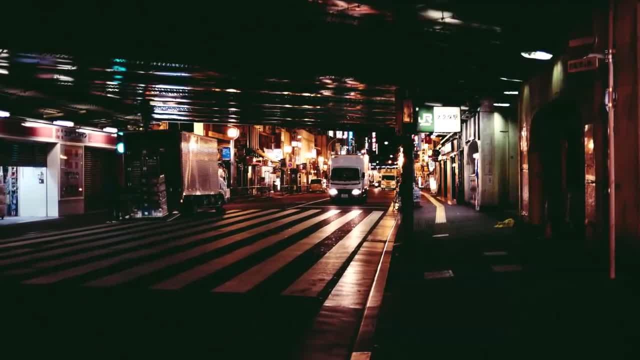 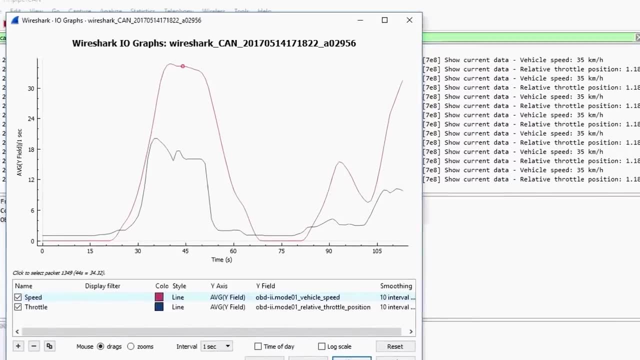 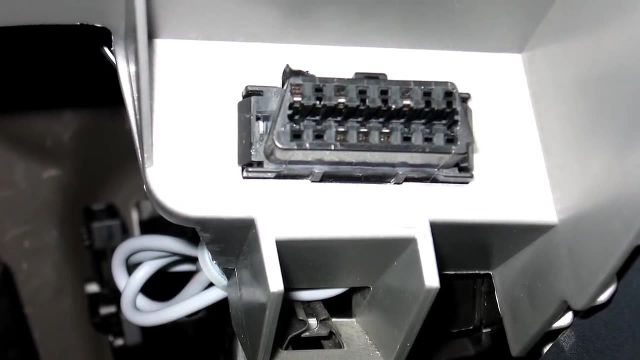 But what makes OBD2 really interesting? OBD2 supports data on many basic real-time parameters, in example, vehicle speed, RPM, fuel consumption. This means that OBD2 is also used for, in example, real-time vehicle telematics or post-analysis using CAN data loggers. 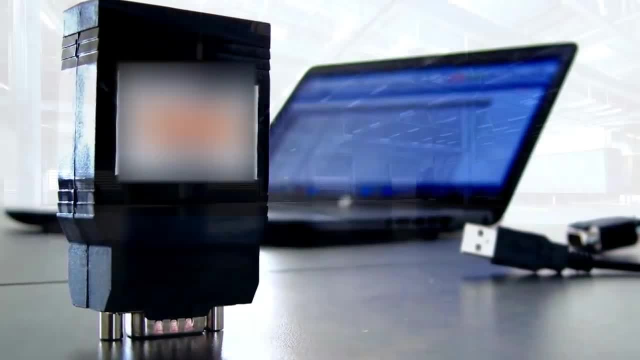 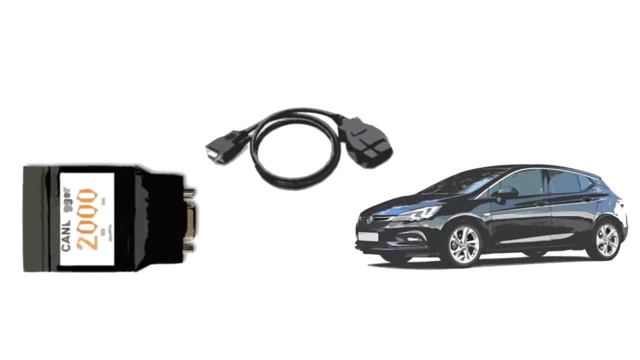 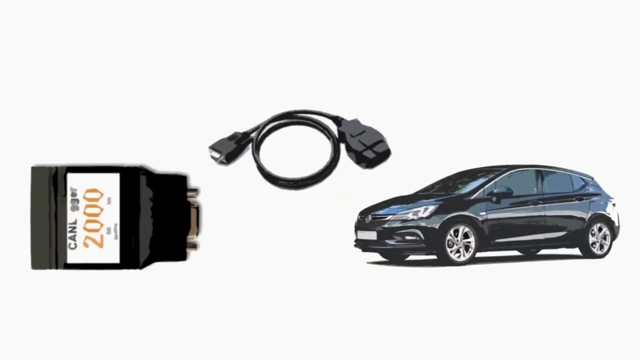 Applications include vehicle fleet management, fuel optimization, proactive vehicle diagnostics and more. To log OBD2 data, the CAN logger must request the data by submitting pre-specified CAN frames with specific parameter IDs to the CAN bus When using the CAN logger. 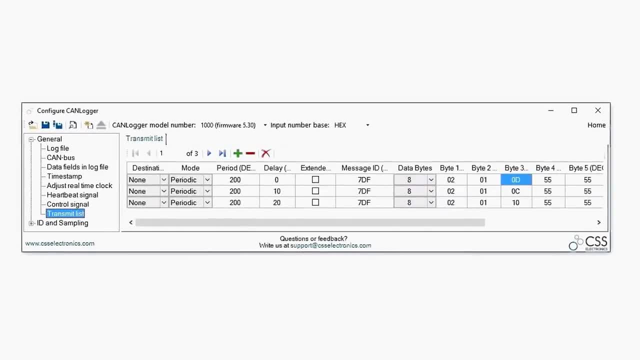 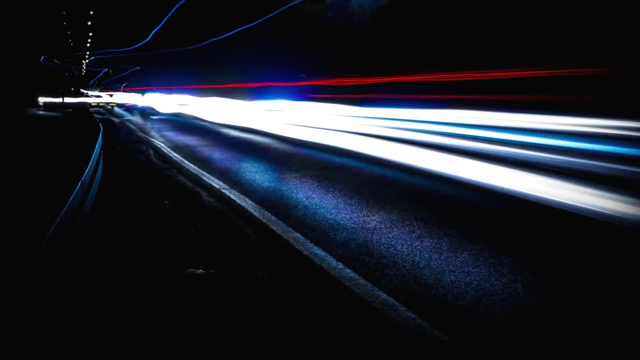 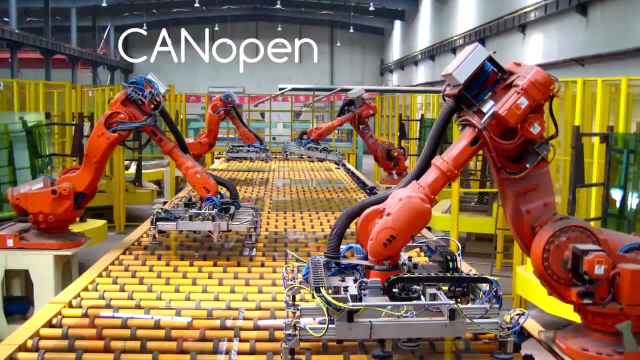 X000, this can easily be configured in CANvus. For basics on OBD2, check out our simple intro to OBD2 or check our practical guides to logging OBD2 data or streaming it in Wireshark- CAN Open. CAN Open is used widely in example. 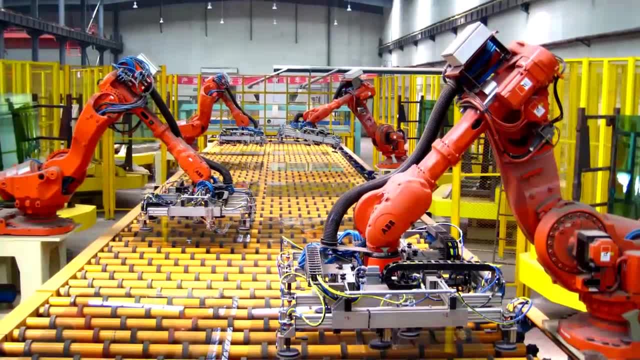 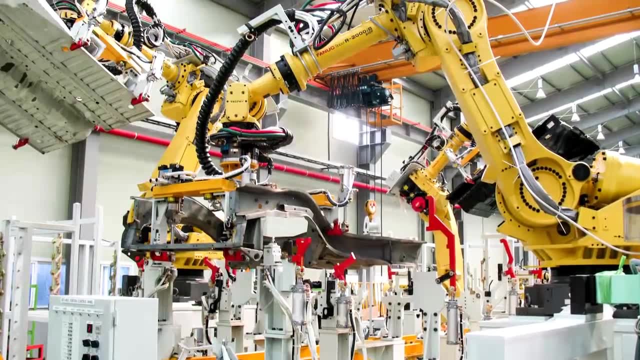 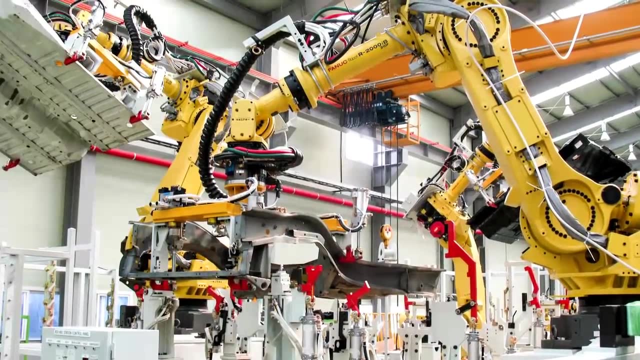 industrial automation applications. It builds on CAN in terms of physical layer- in example, lines, used, voltages- and the data link layer, in example utilizing a CAN frame message based on protocol. In practice, this means that a data logger like the CAN logger X000, is able. 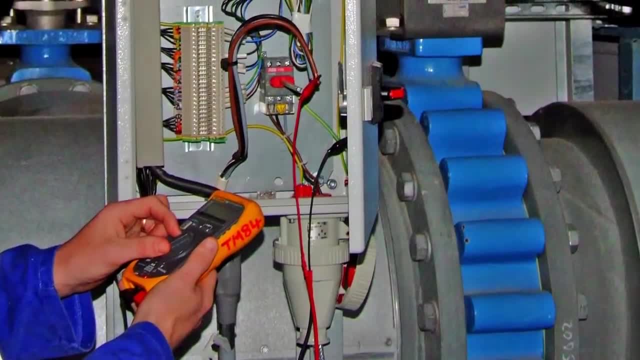 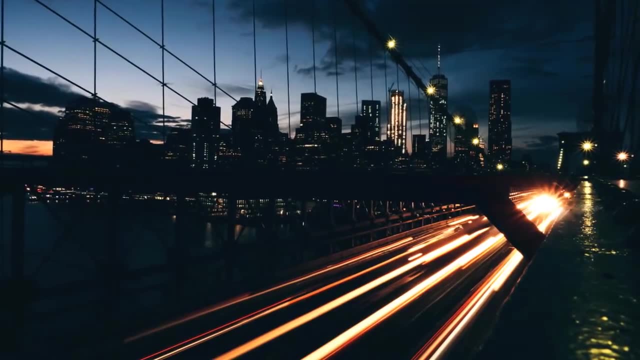 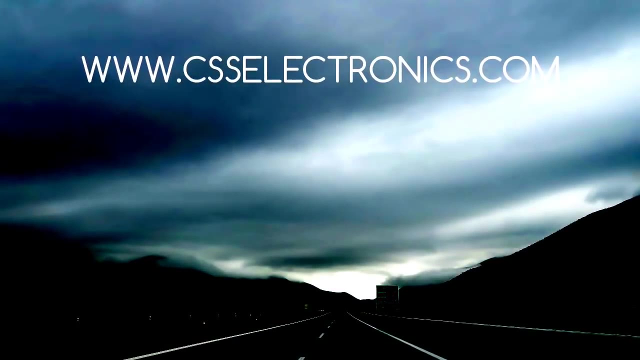 to log data from CAN open applications, though the method of X post data conversion will vary depending on the specific application. Our Intel page contains several intro articles, uses, cases and guides. Let us know if you have more suggestions for the series Interested in our products. Read more about our CAN logger X000. 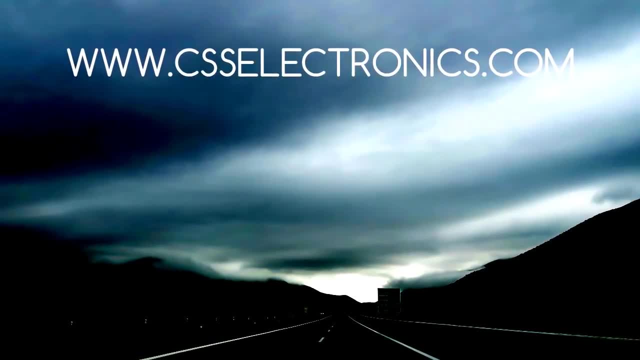 series of CAN bus data loggers here.